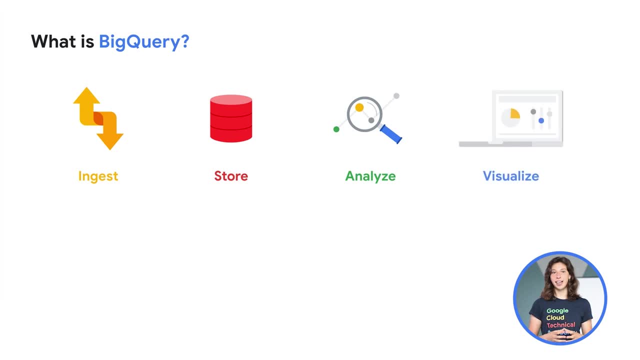 store, analyze and visualize big data with ease. You can simply ingest your data as batch loads or streaming for real-time insights. BigQuery supports both structured and semi-structured data, such as JSON files, for example. With BigQuery, you can store massive datasets- up to petabytes of data. 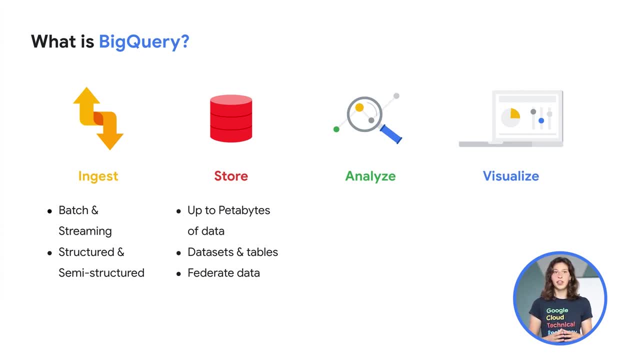 in structured tabular format. There are two different objects to notice in BigQuery: datasets and tables. Tables will be your usual data in tabular format and datasets will regroup those tables as folders To avoid storing duplicates of data. you can also federate BigQuery with other Google Cloud databases. 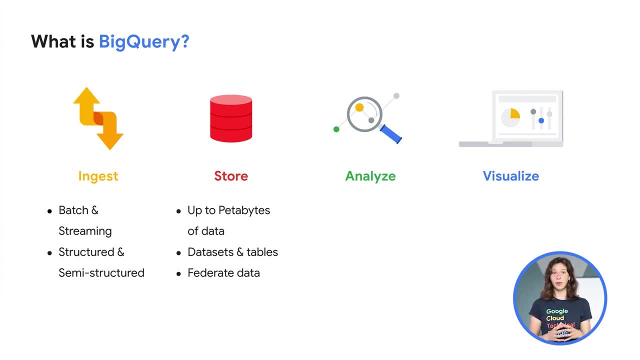 such as Cloud Storage, without copying the data in BigQuery storage, but simply making a connection between products In BigQuery. you can use standard SQL for easy and super-fast querying on massive datasets, for aggregation from different sources and transforming your data with data manipulation. 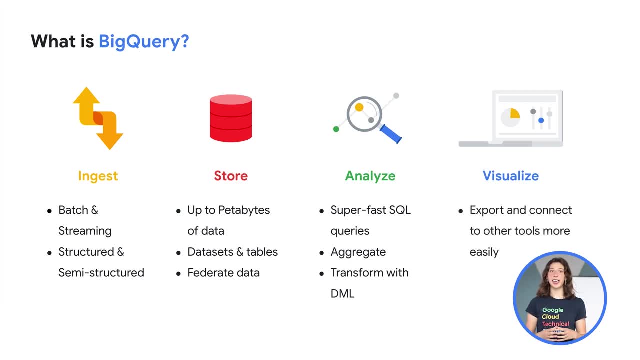 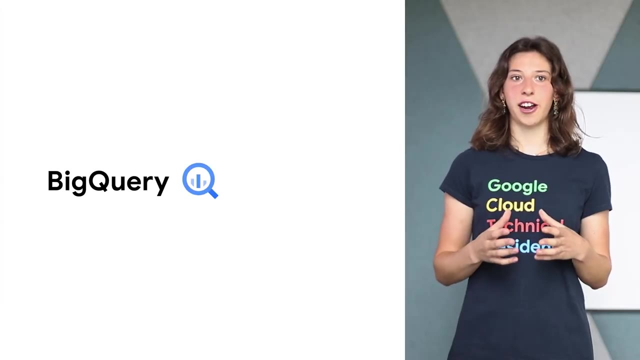 language. Finally, for visualization, BigQuery easily integrates with reporting tools such as Looker spreadsheets, Google's at-no-cost data visualization tool, Data Studio or many other products from our partner ecosystem. Let's dive into the different characteristics of BigQuery. What is BigQuery? 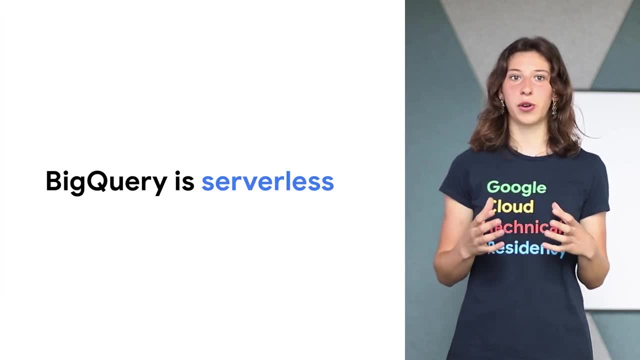 Google BigQuery is fully managed, so you can focus on analyzing your data up to petabyte scale without worrying about the scaling of the underlying infrastructure. Google BigQuery is ML predictive, enabling your data scientists or analysts to build and operationalize ML models. With only a few lines of SQL, you can train and execute your models on data. 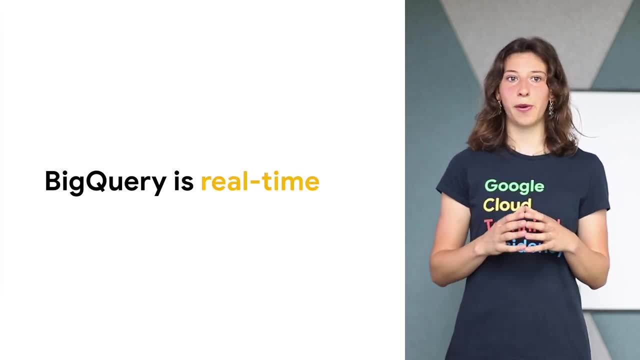 analysis without needing to move it around. Google. BigQuery is real-time Stream data and accelerate business decisions by getting your analysis on the spot. BigQuery is multi-cloud and with BigQuery Omni, you can ingest and analyze data from other cloud providers. 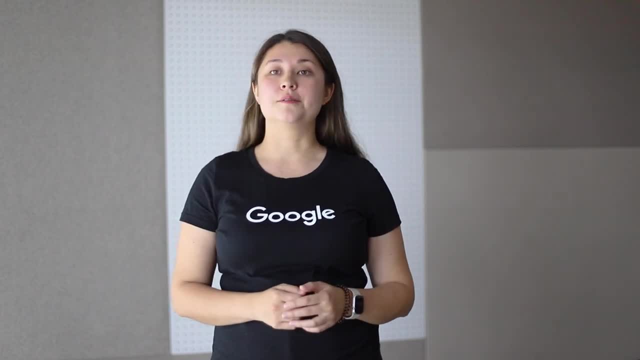 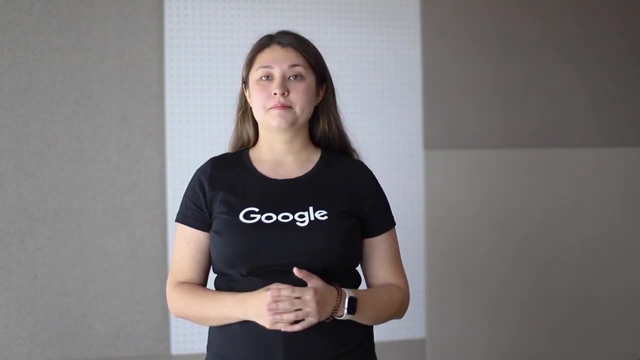 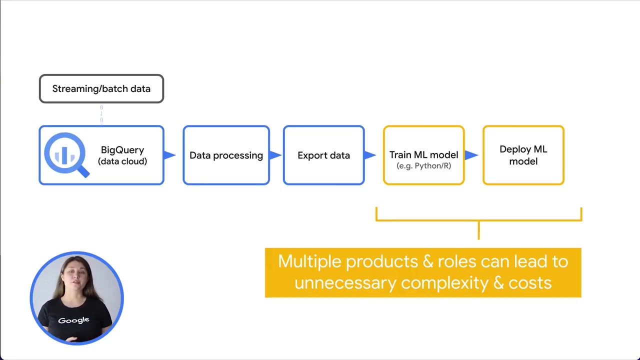 As we learned, BigQuery is a great tool when it comes to data analysis and enables users with quick access to data insights with no extensive programming skills. But what about large data sets, management and machine learning? As you know, both require knowledge of ML frameworks. Quite often, this excludes data. 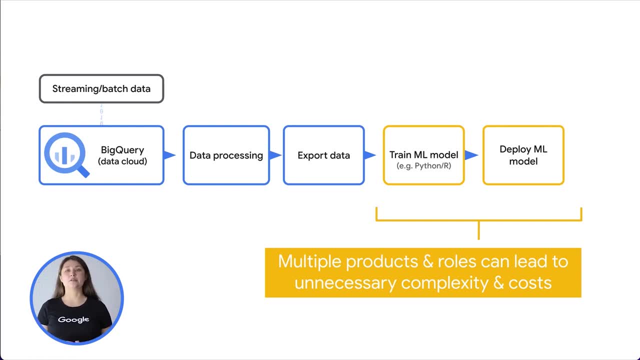 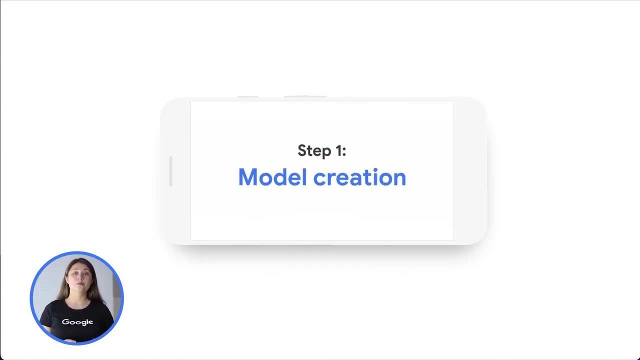 analysts who understand the data but have limited ML knowledge and programming expertise. BigQuery ML empowers data analysts to use machine learning through existing SQL tools and skills Without needing to move your data out of BigQuery. with BigQuery ML, you can train and deploy machine learning models directly using SQL. 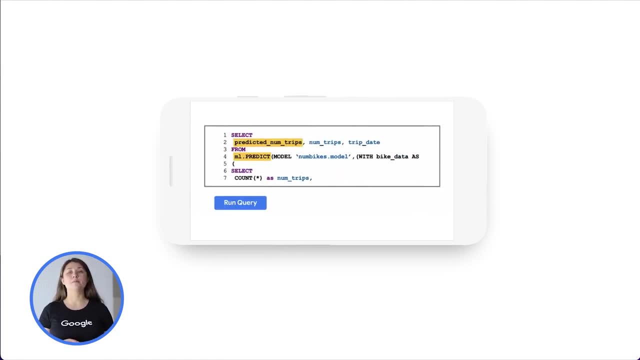 BigQuery ML takes care of data extracting, model training and deploying. for you, That means you've got data storage, data analytics and machine learning all within BigQuery. As your business data keeps growing in volume over time, your data analytics pipeline has to. 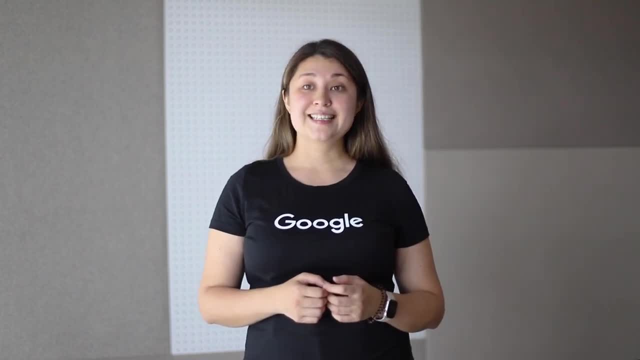 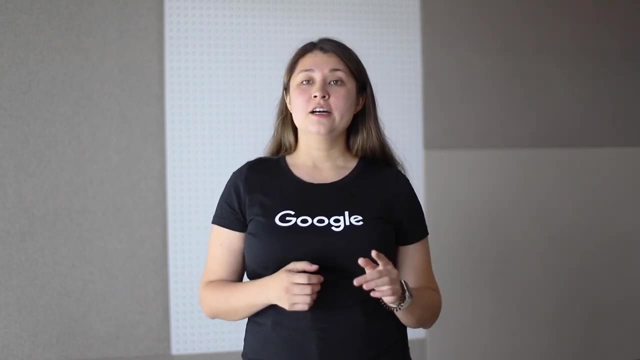 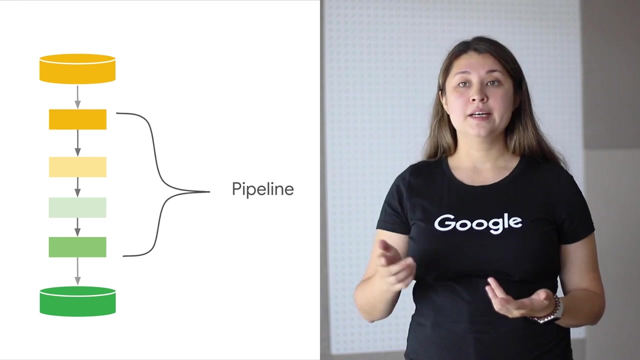 be scalable to adapt to the rate of change. Let's see how BigQuery can help us build an ETL pipeline to accommodate the scale. But first let's define what is a pipeline and what does ETL mean. A data pipeline is a series of data processing steps. Each step delivers an output. 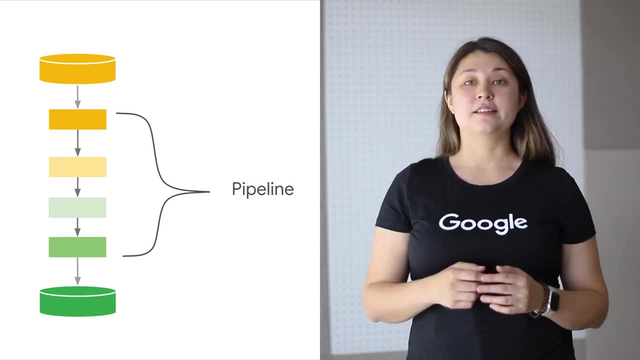 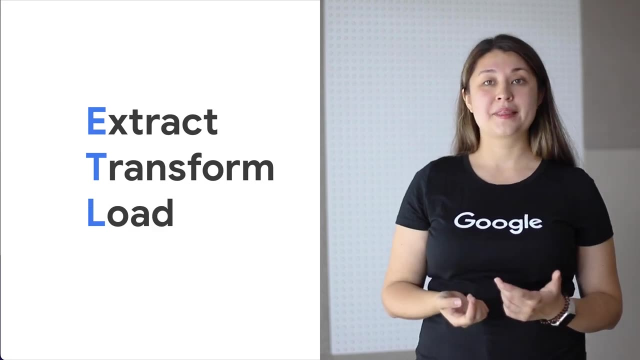 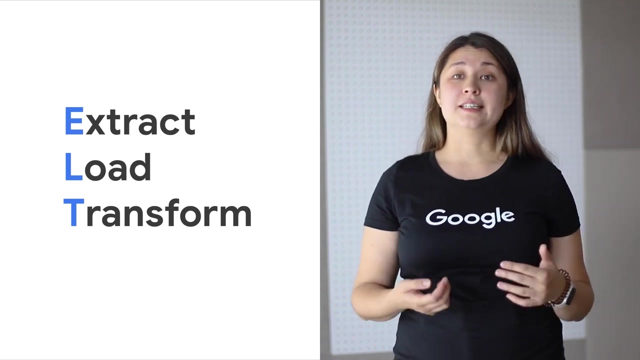 that is an input to the next step. ETL refers to a specific type of data pipeline And it stands for extract, transform and load. Another popular pattern is ELT: extract, load and transform. The transformation can be done inside of BigQuery. Extract refers to pulling data out of source. 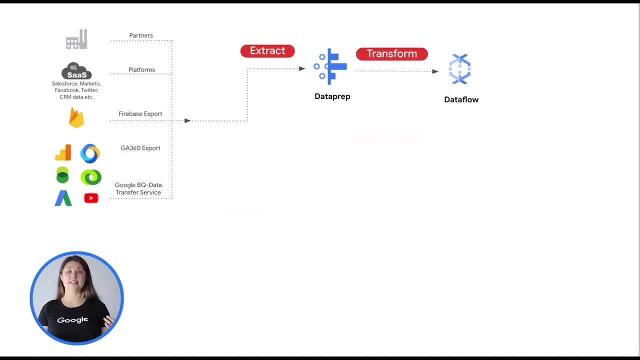 about modifying the data so that it can be loaded into the destination, and load is about inserting the data into the destination. this is a common way for organizations to combine data from multiple systems into a single data warehouse. etl can be used to store legacy data or, as more typically, 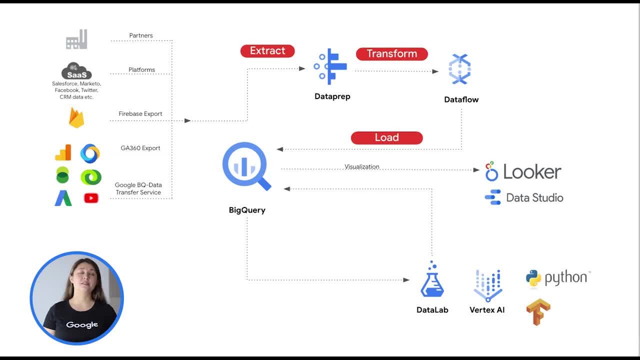 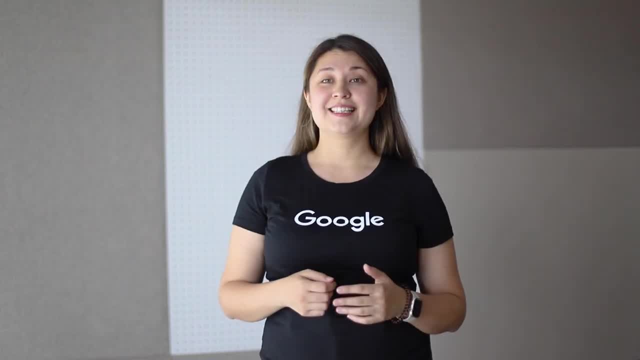 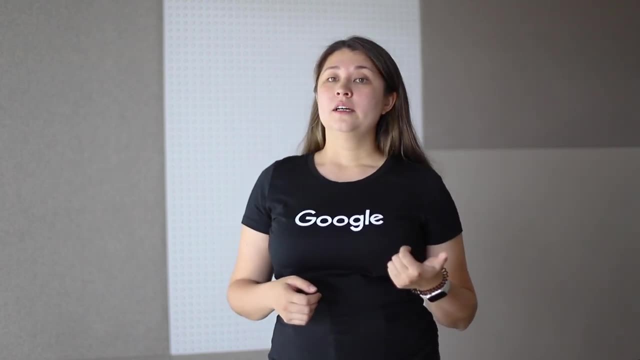 today aggregate and process data to analyze and drive business decisions. bigquery is a great choice for your etl data pipeline. let's take a look at the architecture components of an etl solution for google bigquery using google cloud data flow, google cloud pops up and google cloud. 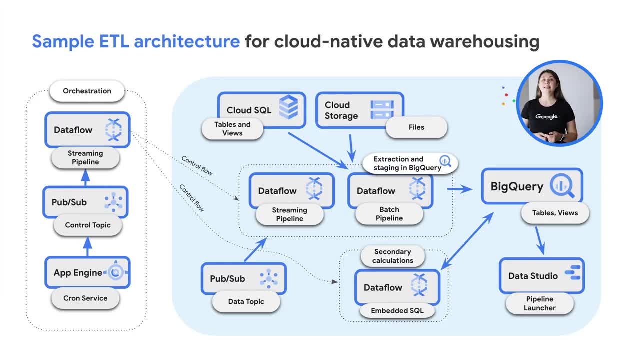 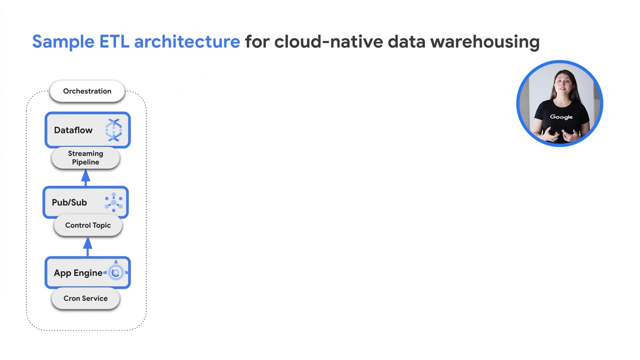 up engine chrome as building blocks. as an example, we can build a task orchestrator using google up engine chrome service, google cloud pops up control topic and google cloud data flow in streaming mode. then we will be using google cloud data flow for importing bounded batch row data from sources such as relational google cloud. 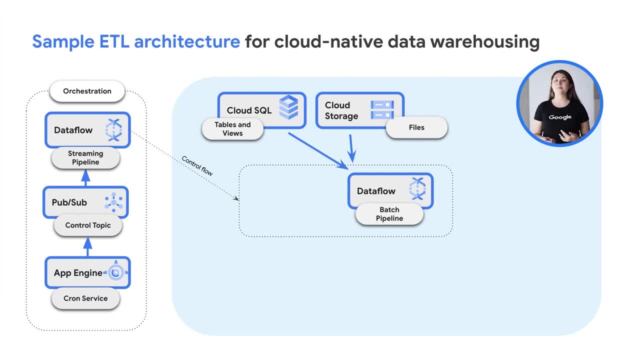 sql database, for example mysql or postgresql, we as a gdbc connector and then we will be storing the files in google cloud storage. then google cloud data flow will be used for importing unbounded streaming data from google cloud pops up data ingestion topic and after that bigquery. 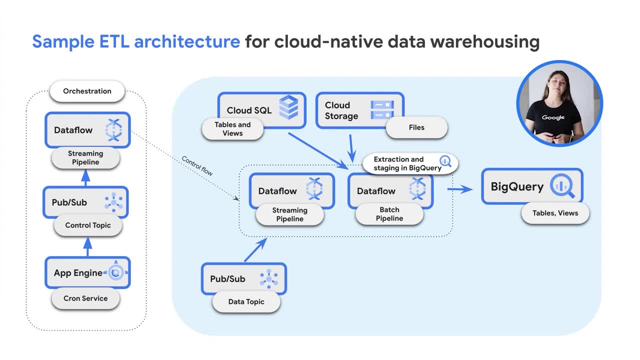 will be used for storing staging in final data sets. an additional etl transformation will be enabled via google cloud data flow and md sql statements. an interactive dashboard in data studio can be connected to bigquery just to visualize your data insights. all these components are examples of fully managed services. 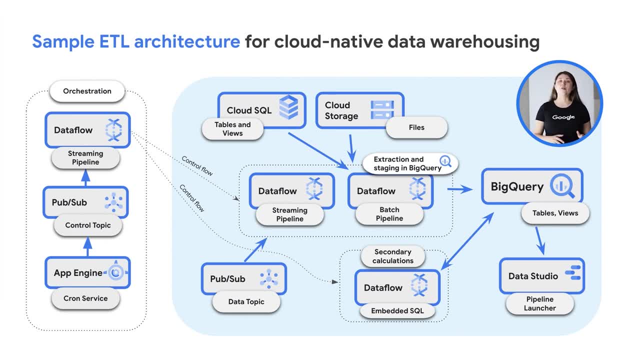 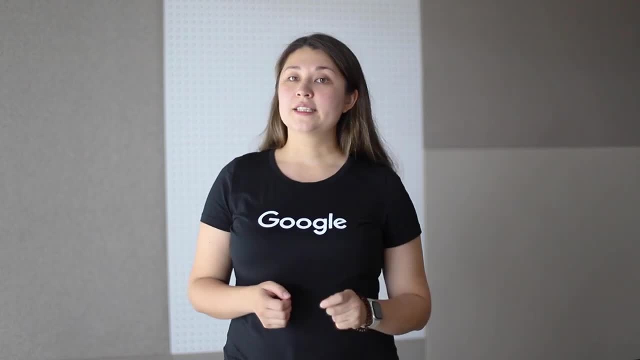 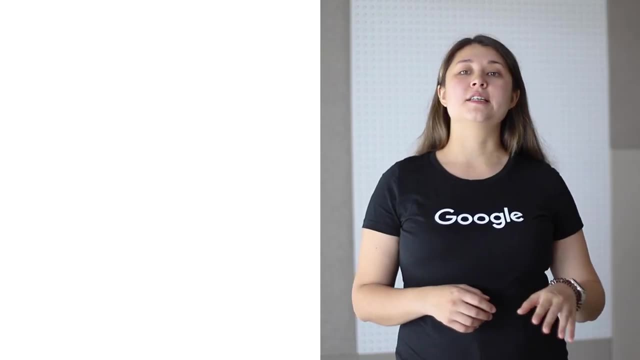 on google cloud platform. with this architecture, there is no infrastructure for you to deploy, manage, secure or scale, and you only pay for what you use. when it comes to data lifecycle management, it's important to take into account the data governance principles. data governance is everything you do to ensure your data is secure. 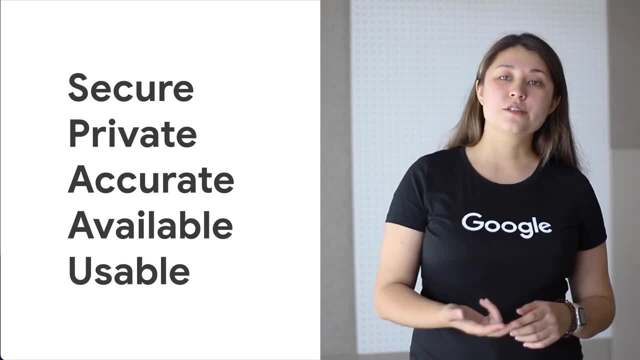 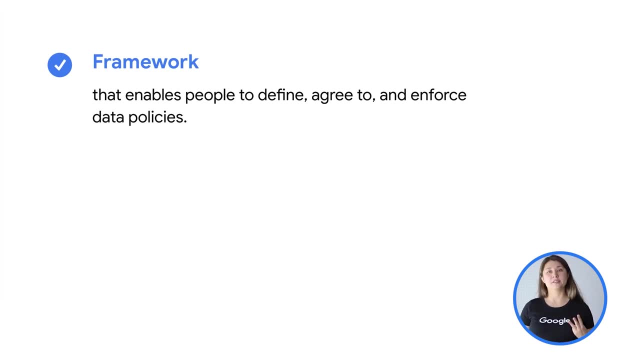 private, accurate, available and usable inside your data warehouse. we recommend that you build your data governance practice around three key components: choosing the right framework that enables people to define, agree to and enforce data policies. creating an effective process for control, oversight and administration over all data assets across on-prem. 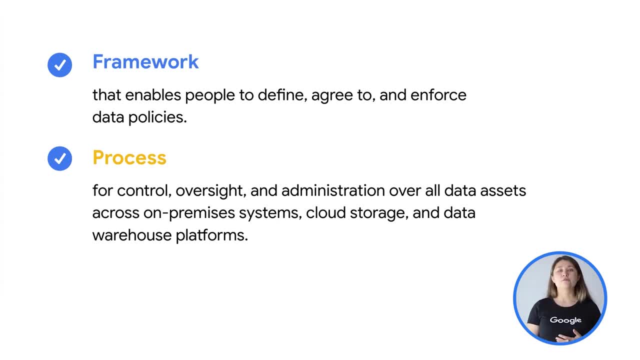 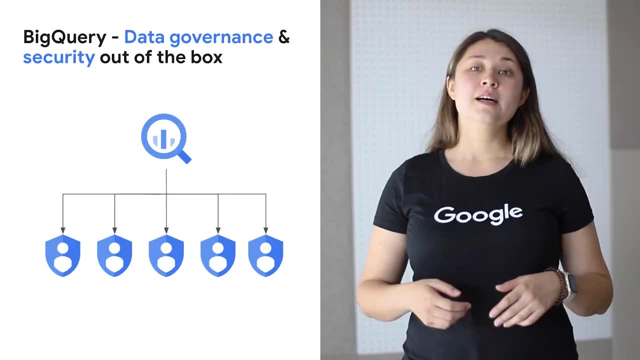 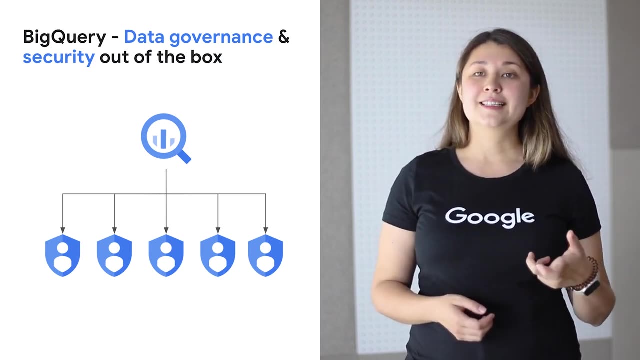 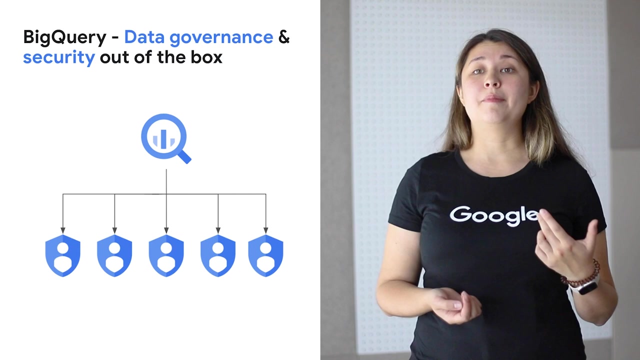 cloud storage and data warehouses platforms and, of course, choosing the right tools and technologies for overseeing and supporting data policy compliance. bigquery offers built-in data production at scale. within bigquery, users can assign data set level and project level permissions to help govern data access. Also, we have data encryption set by default. 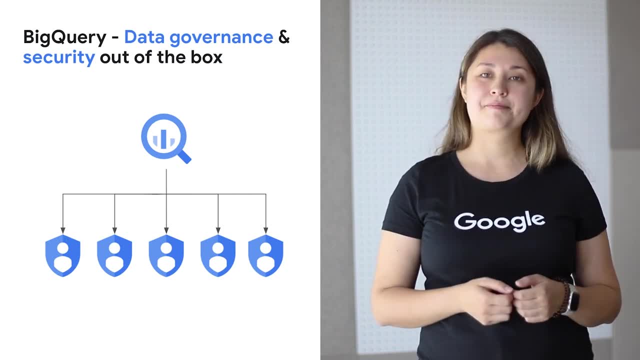 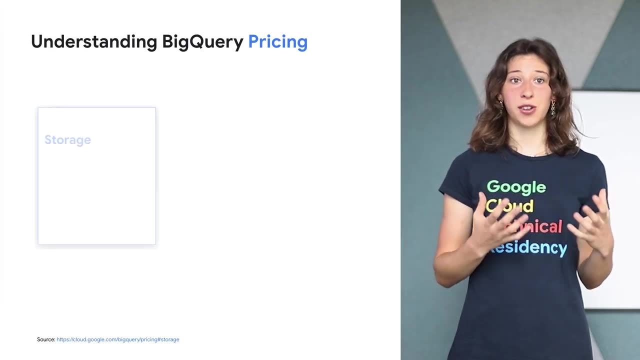 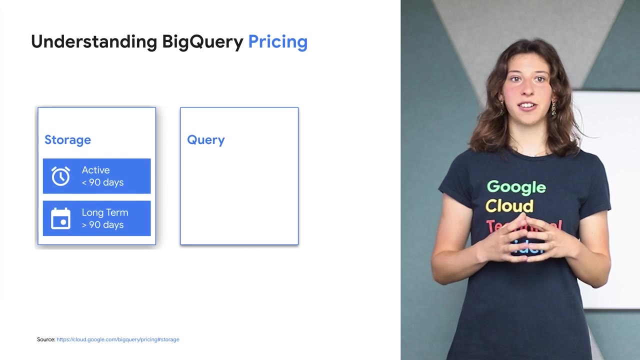 to ensure data security at all levels. So what does it cost you to use BigQuery? Let's take a look at pricing. You pay for storage queries and some ingestion and export use cases. Storage costs are based on the amount of data stored. 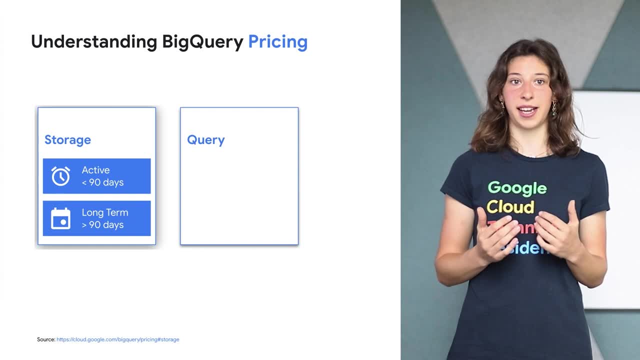 and has two rates based on when the data was modified for the last time. Tables or partitions in long-term storage, meaning that they weren't modified in the last 90 days, see their storage price drop by 50%. Query costs are either on-demand: 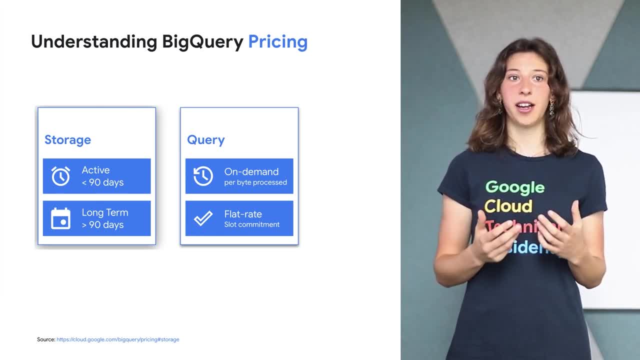 meaning that you'll be charged for the number of bytes processed by query. the first terabyte processed is offered- or flat rate. With flat rate, you purchase dedicated processing capacity to run queries at a reduced price. Those resources are called slots. They are virtual CPUs. 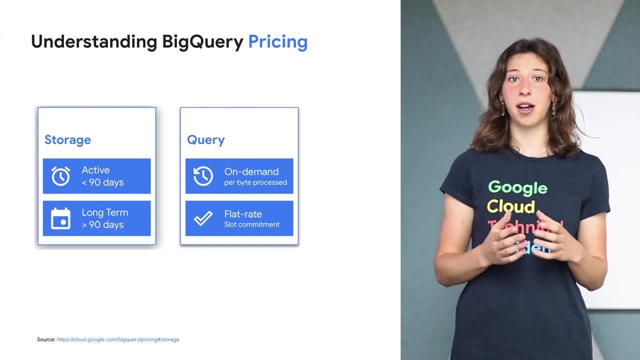 With flat rate. you can make commitments by the second, the month or the year. The rule of thumb is that you should consider flat rate once your BigQuery processing cost exceeds $10,000 of budget. Note that you are not charged for queries that return an error. 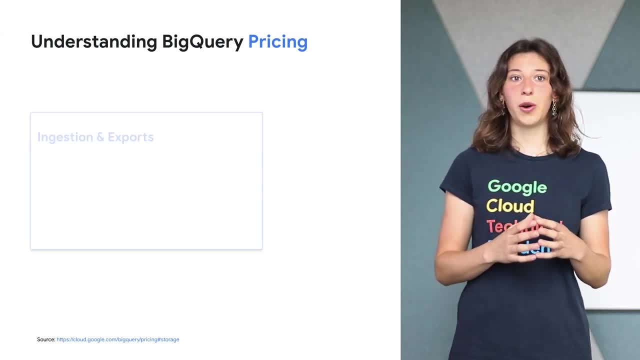 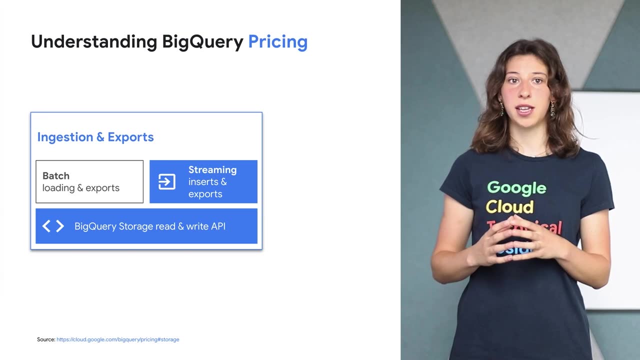 or for queries that retrieve results from the cache. Loading and exporting batch data to BigQuery is at no cost. You'll be paying for streaming, inserts and exports and the use of the BigQuery API. You can find the link to detailed pricing in the description. 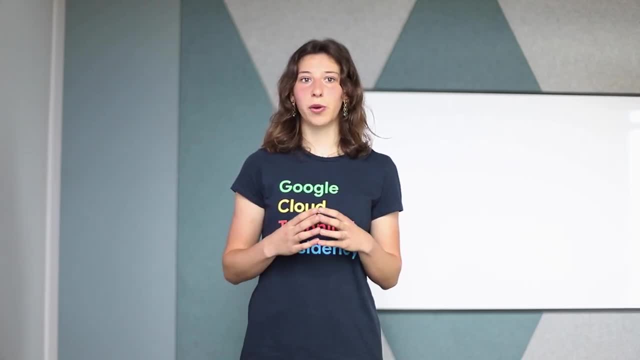 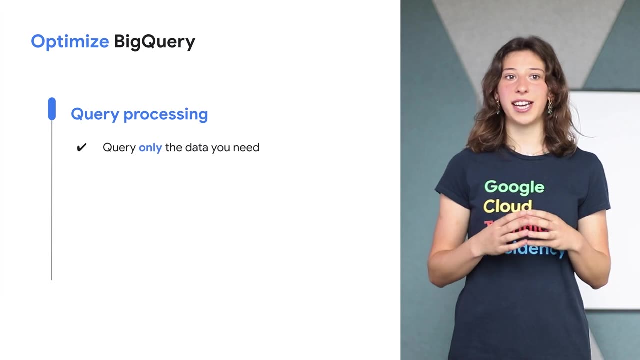 And what about performance and cost? There are several ways to optimize them in BigQuery. Let's start with query processing. You should only query the data you need. First use the preview option to explore your data before you write a query. It's free. 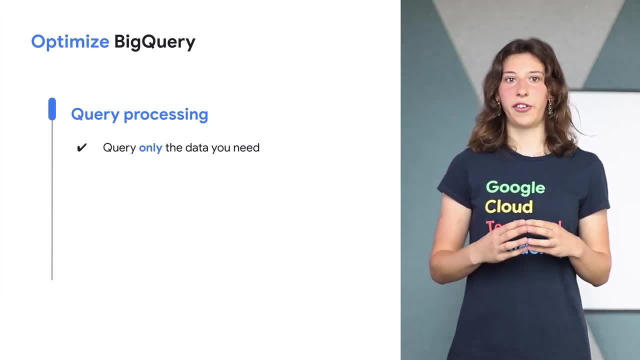 When you write a query, avoid the SELECT ALL statement. Filter your query as early and as often as possible, And avoid SQL anti-patterns such as joins that generate more outputs than inputs. Finally, check how much your query is going to be charged by seeing the number of bytes processed. 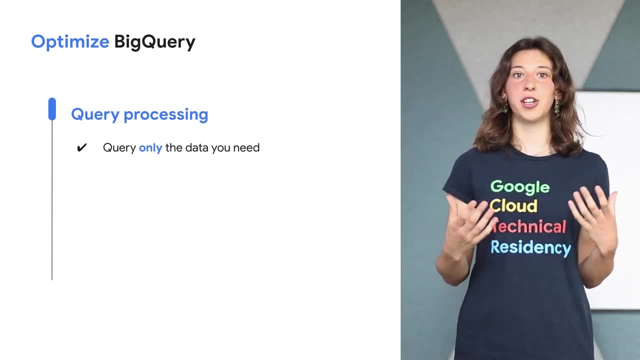 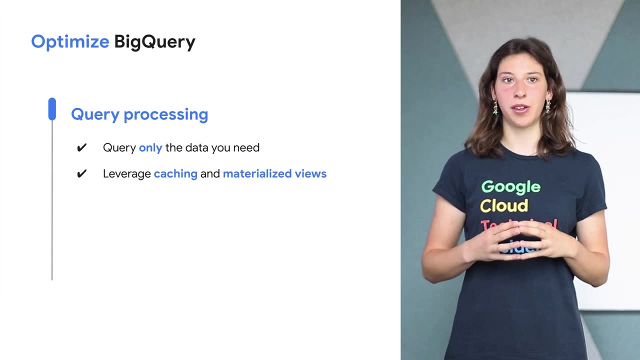 in the UI or do dry runs to get an estimation of your costs. Use cache intelligently. BigQuery writes all your query results to your table. You either explicitly identify the destination table or it is cached as a temporary table. Temporary cached results tables are: 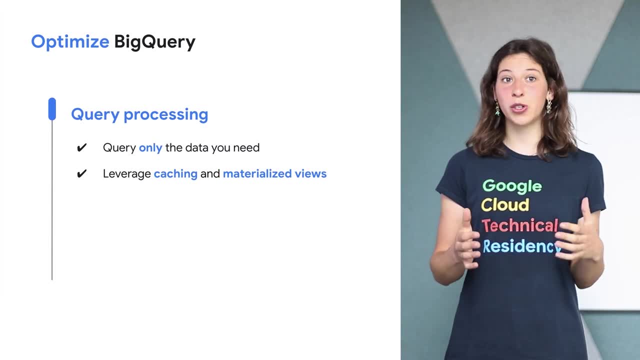 maintained per user, per project. There are no storage costs for temporary tables. Enforce cost controls to avoid human errors. Enforce max limits on bytes processed per query or at the user and project level. Partitioning and clustering your tables improves query performance and can help reduce costs. 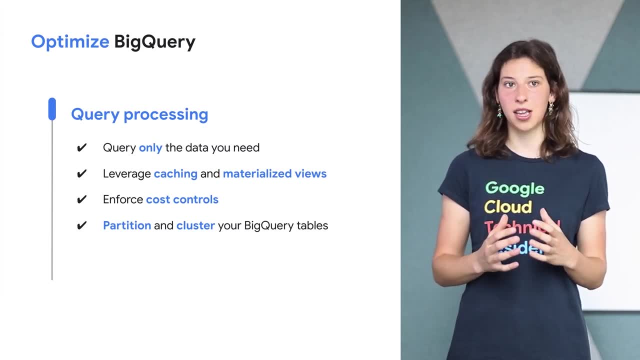 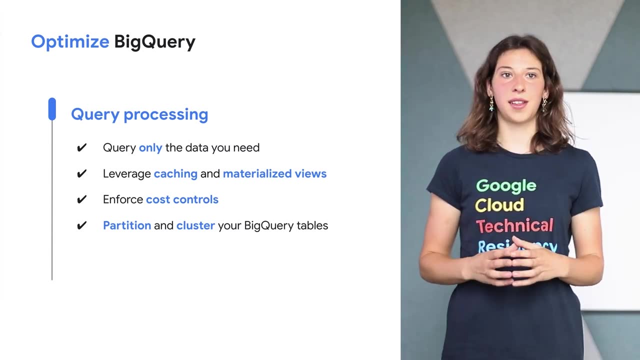 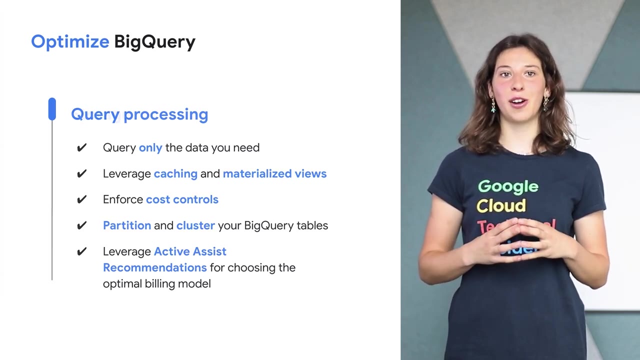 by reducing the amount of data processed by queries. You can partition by ingestion, time, date, timestamp or integer range, For example. Active Assist recommendations guide you through the optimal billing model based on your usage. The BigQuery slot recommender helps on-demand customer. 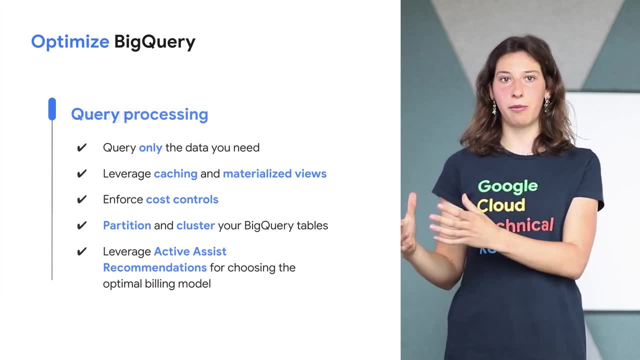 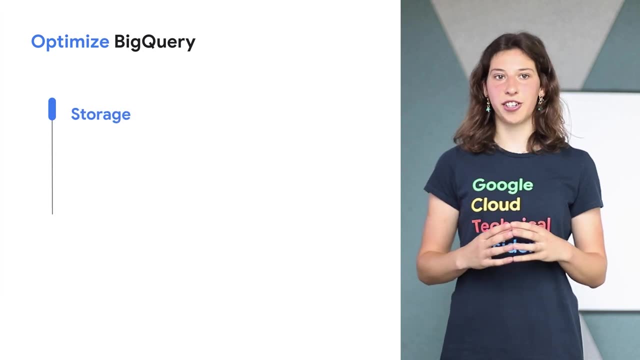 estimate the number of slots when migrating to a flat rate pricing, and does so by providing four options on a cost performance scale. Concerning storage, keep in mind to enforce data retention policies by setting up expiration at the data set table or even the project. 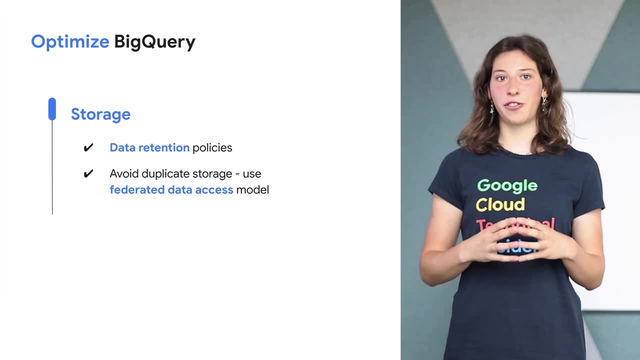 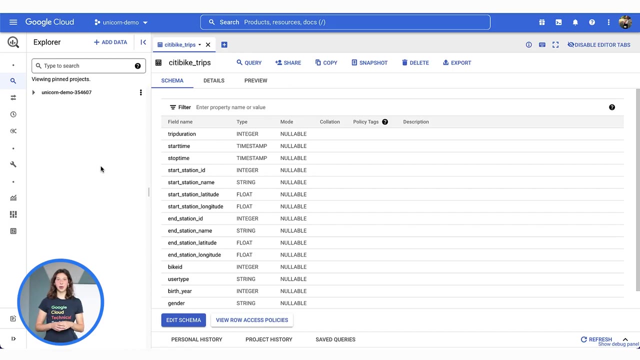 Partition level. Also, make sure you leverage federated data access. You can avoid duplicate copies of data by connecting BigQuery to Google Cloud Storage and avoiding BigQuery storage costs. Now let's take a quick tour to the console. In this demo, we will explore a public data. 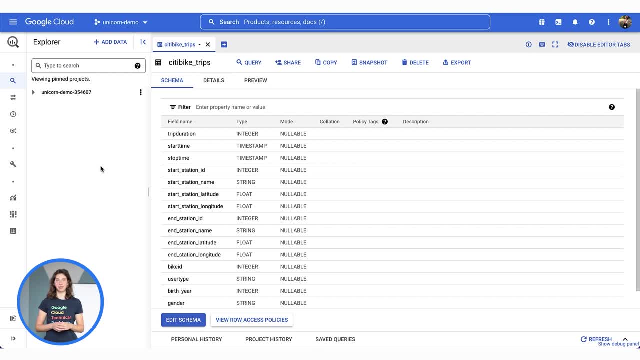 sets for New York City City Bike trips In BigQuery. the year I keys as follows. Here I can see my project, I can click on my data set and my data set here contains two tables: City Bike Stations and City Bike Trips. 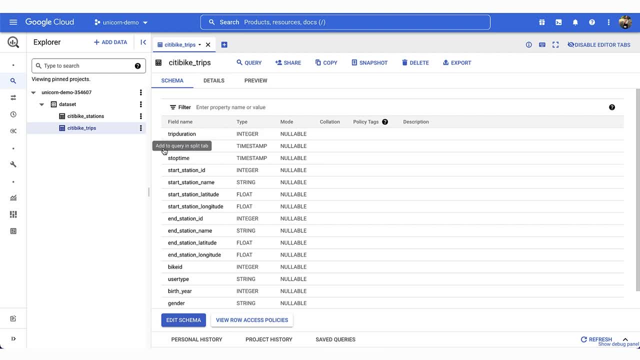 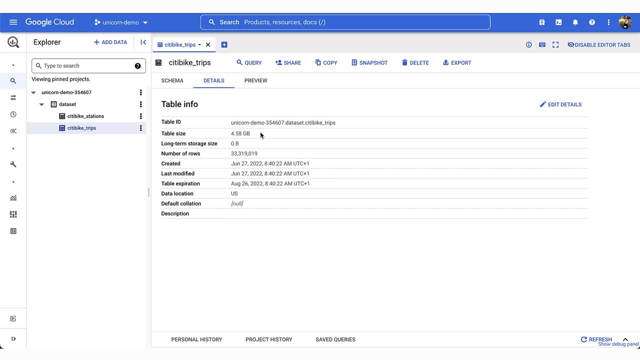 I can visualize the schema of a table which gives me the different columns, their type and their description In details. I can view the size of a table and the number of rows. Here you can see we have a large data set of more than 33. 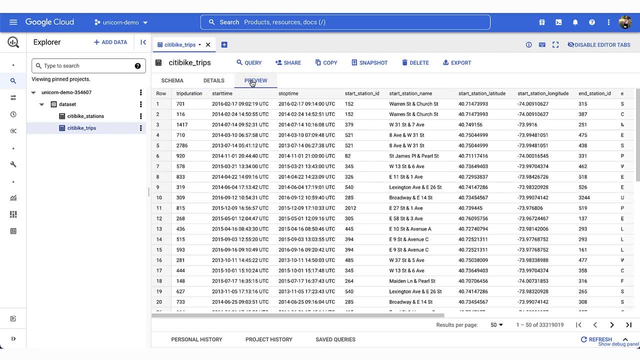 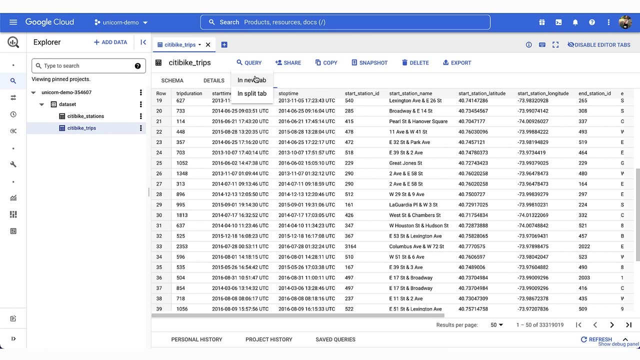 million rows. The preview window- and this is my favorite feature- allows you to visualize a part of the table and see what the data looks like without performing any query. Let's try to do a query now. It is very straightforward: You simply have to click on the Query button. 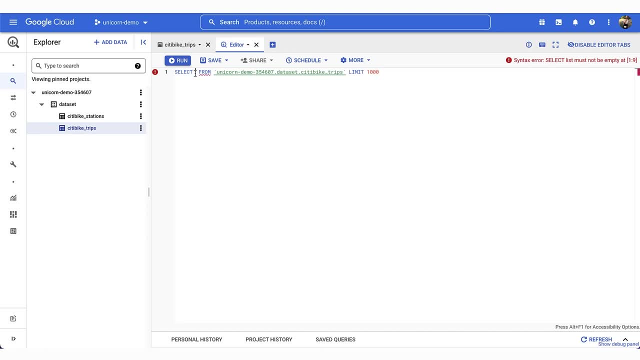 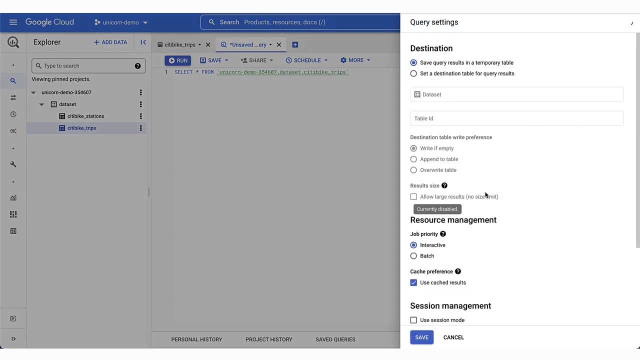 and compose your query with SQL language. So here I'm going to query the whole table. I am going to disable the cache so you can see how long it takes to query the whole table In BigQuery. you can see that the query table is very simple. 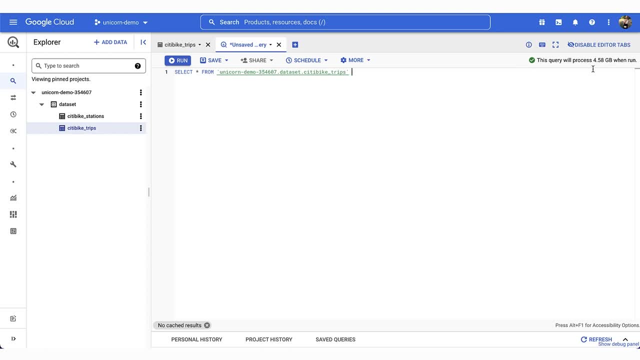 You can see how long it takes to query the whole table In BigQuery. you can see how long it takes to query the whole table. You can also visualize the number of bytes BigQuery will process with your query so you can keep an eye on billing. 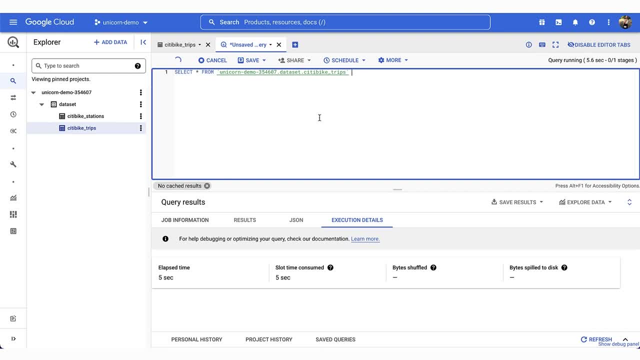 So here let's wait and see how long it takes for BigQuery to query the whole 33 million row table. So here, as you can see, it only took 29 seconds to query the whole table, All right. So here let's do another query and see. 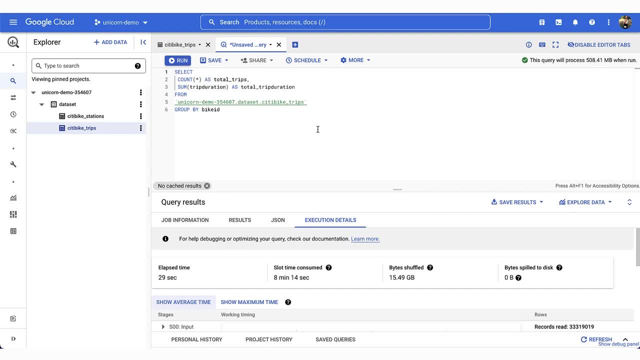 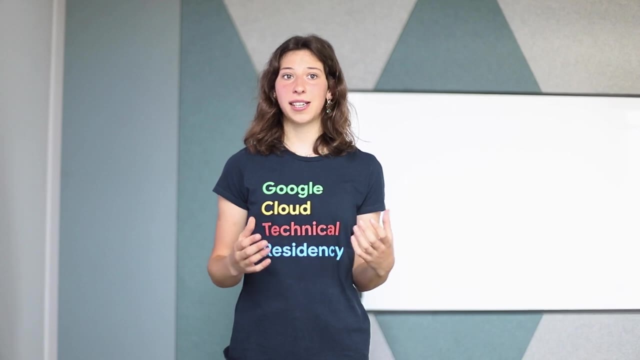 how fast BigQuery is for more complex queries. As you can see, as soon as you group or add a condition, both the duration and amount of bytes shuffled dramatically decrease. You can perform any and very complex SQL query. you want to make your analysis and extract your insights. 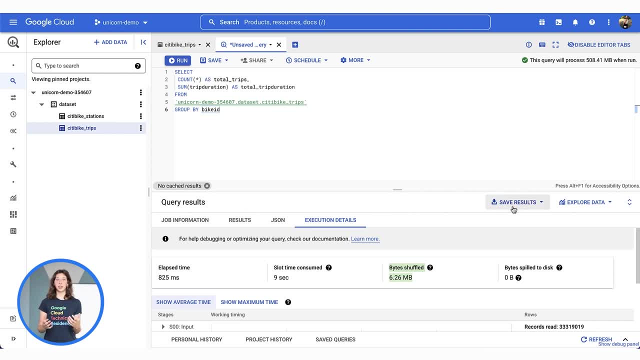 Once you have gathered the information you need, you can save your query. You can also export the results either in another BigQuery table, Google Sheets or a CSV or JSON file to share externally within your drive or through a local file. 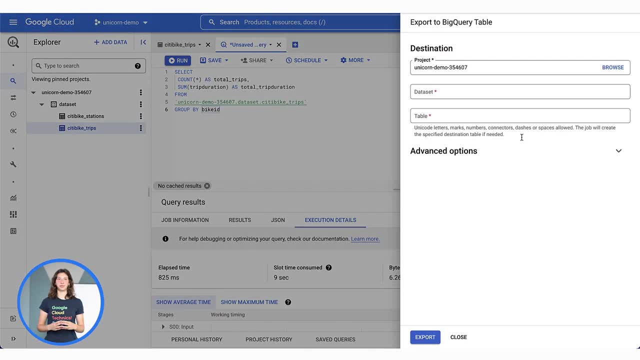 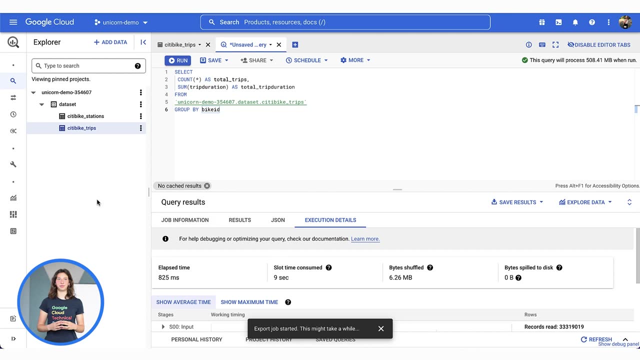 Let's export our results to a BigQuery table. I can now see the table added to my data set and my project. The location of your table will be the same as before. The location of your table will be the same as before. It will be the one of your data set by inheritance. 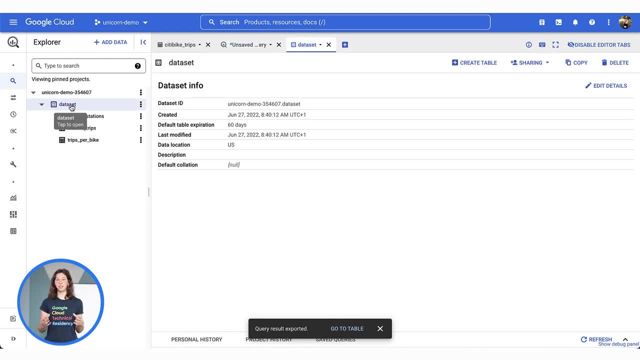 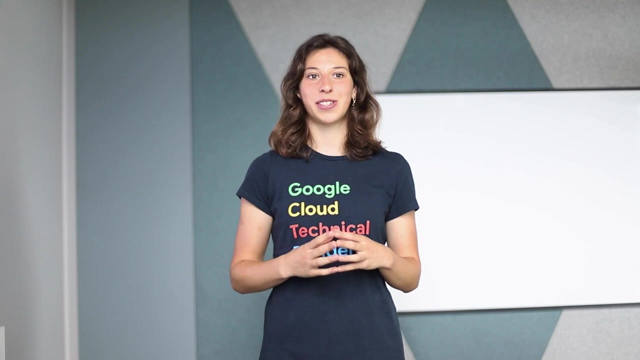 The data set can be located in a specific region- London, or a multi-region, larger geographic area like the US. Location of your data is an important concept for query processing and loading and extraction of your data. Be sure to try BigQuery Sandbox. 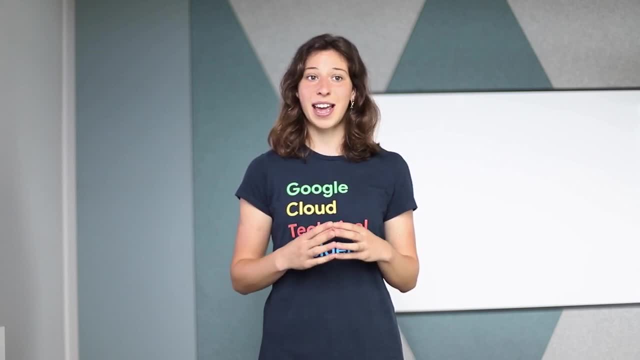 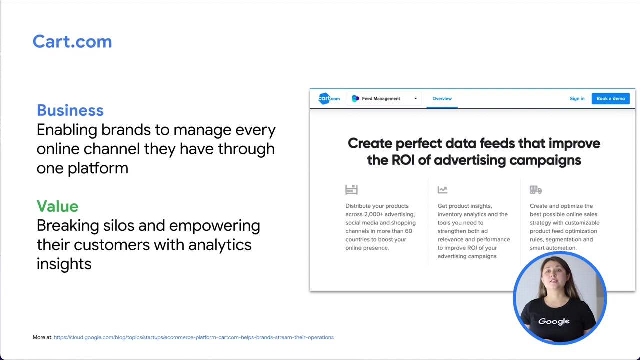 It lets you explore BigQuery capabilities at no cost and confirm that it fits your needs. The Sandbox lets you experience BigQuery without providing a credit card, creating a billing account or enabling billing for your project. And if you wanted to see a real-life example, 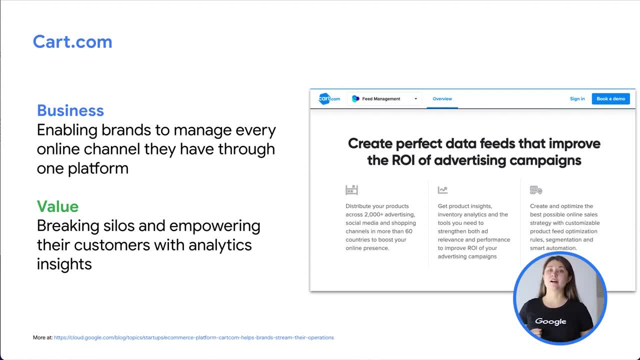 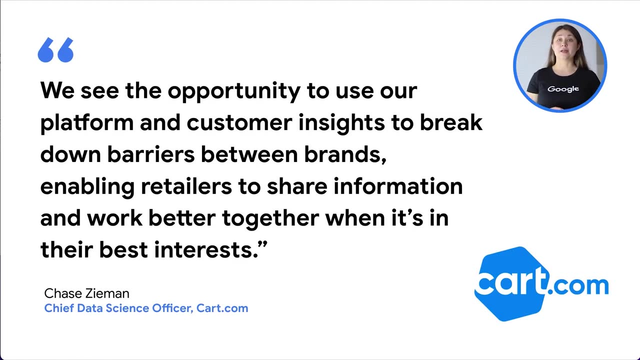 of a BigQuery power in action. let's take a look at Cardcom, an e-commerce platform which helps to democratize e-commerce by giving brands of all sizes the full capabilities they need to take on the world's largest online retailers. Supported by the startup program by Google Cloud and Google. 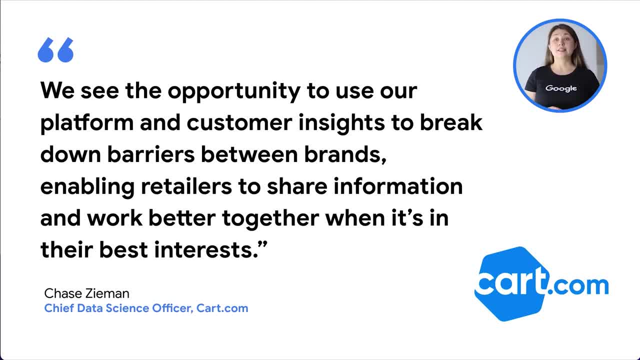 Cloud Solutions. Cardcom is the largest online retailer in the world. Their end-to-end environment empowers retailers to keep more of their revenue, set up proven strategies for managing all aspects of their business and act on meaningful insights from customers' data every step of the way. 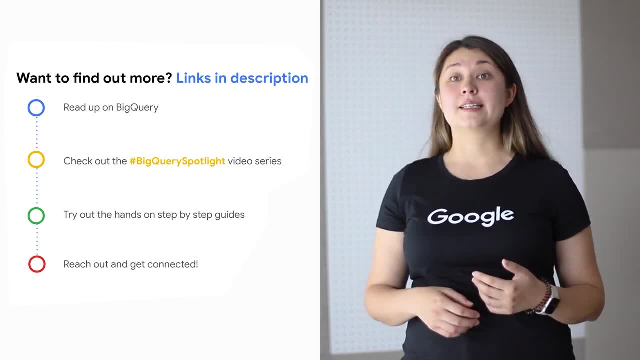 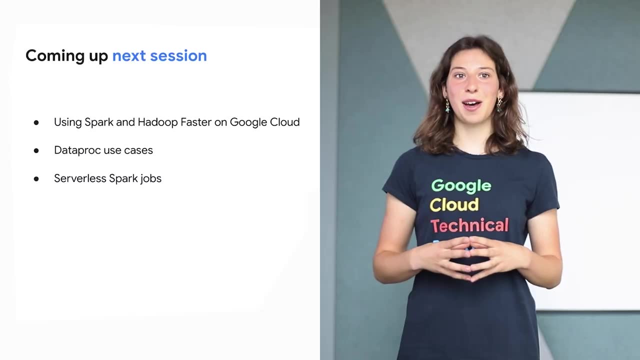 So, all in all, BigQuery is a go-to solution when it comes to getting insights from your data. We hope that this has given you a good understanding on how you can get started on BigQuery Coming up in our next session, we'll